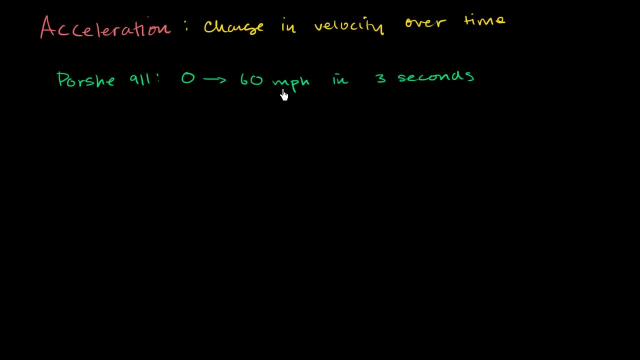 to the east in 3 seconds. So what was the acceleration here? So I just told you the definition of acceleration. It's a change in velocity over time. So the acceleration- and once again acceleration- is a vector quantity. You want to know, not only how much. 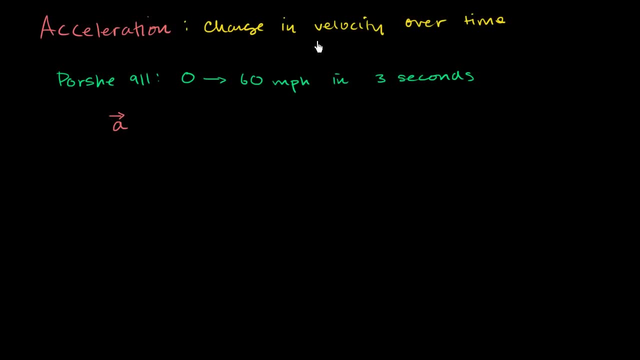 is velocity changing over time. you also care about the direction. It also makes sense because velocity itself is a vector quantity. It needs magnitude and direction. So the acceleration here, and we're just going to assume that we're going to the right. 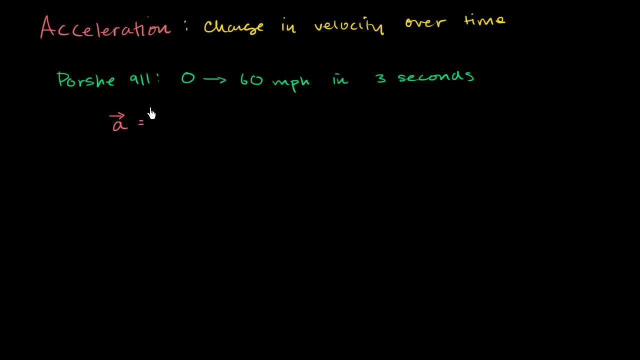 0 to 60 miles per hour. 0 miles per hour and 60 miles per hour to the right. So what is the? it's going to be change in velocity, So let me just write it down with different notation, just so you can familiarize yourself, if you see it. 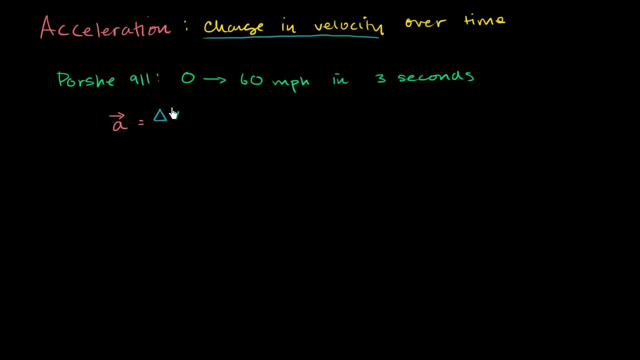 in a textbook this way. So change in velocity, This delta symbol right here- just means change in, Change in velocity over time, And it's really, as I've mentioned in previous videos, time is really a change in time, But we could just write time here. 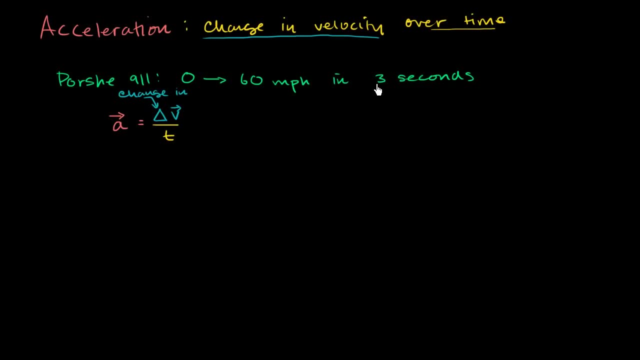 This three seconds is really a change in time. It might have been if you looked at your second hand. it might have been five seconds when it started and then it might have been eight seconds when it stopped. So it took a total of three seconds. 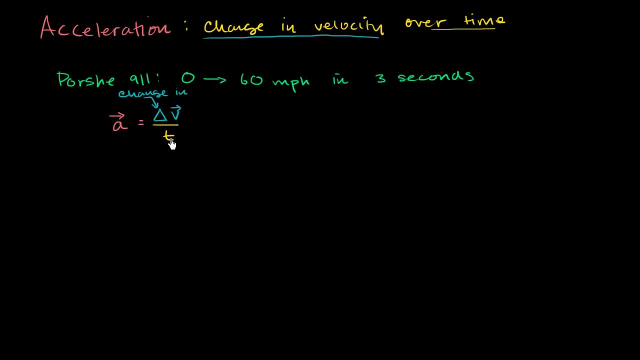 So time is really a change in seconds, But we'll just go with the time right here or just with the t. So what's our change in velocity? So our final velocity is 60 miles per hour. Our final velocity is 60 miles per hour. 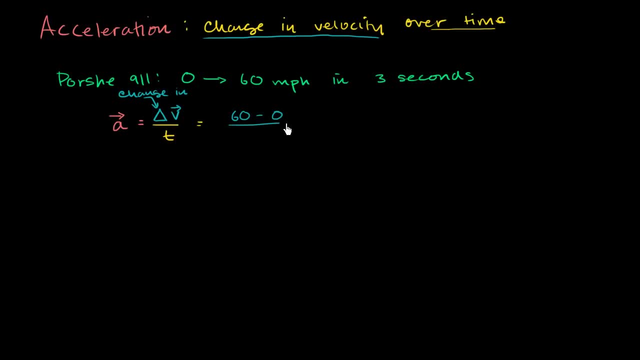 And our original velocity was 0 miles per hour. So it's 60 minus 0 miles per hour. And then, what is our time? What is our time over here? Well, our time is, or we could even say our change in time. 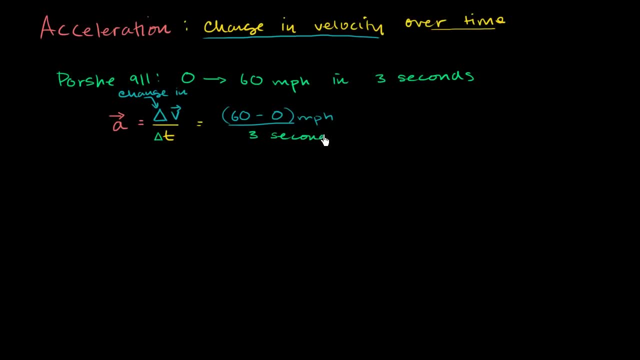 is three seconds, So this gives us 20 miles per hour per second. Let me write this down So this becomes This top, This bottom part, is 60.. 60 divided by 3 is 20.. So we get 20.. 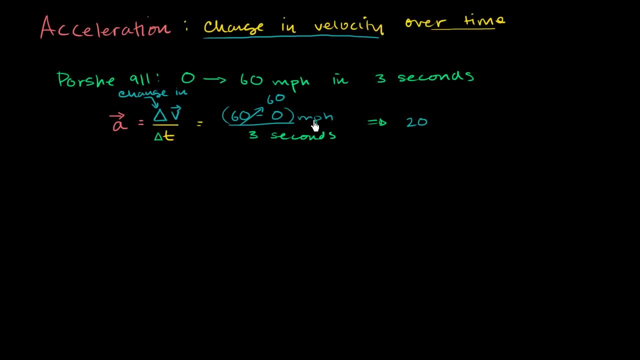 But then the units are a little bit strange. We have miles. Instead of writing mph, I'm going to write miles per hour. That's the same thing as mph. And then we also in the denominator right over here have seconds, which is a little bit strange. 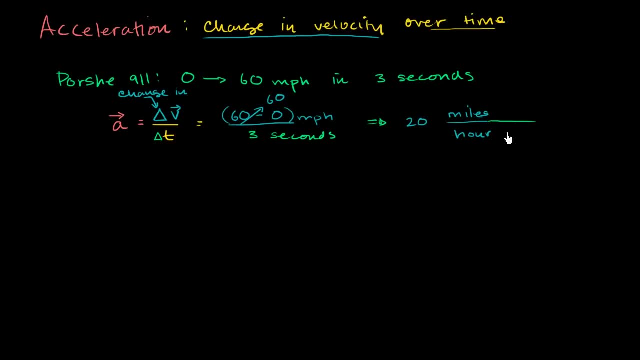 And, as you'll see, the units for accelerating do seem a little bit strange, But if we think it through it actually might make a little bit of sense. So, miles per hour, And then we could either put seconds like this or we could write per second. 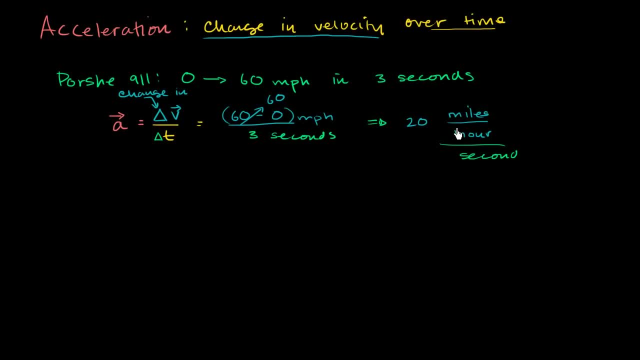 And let's just think about what this is saying, And then we could get it all into seconds, or we could all get into hours, whatever we like. This is saying that every second, this Porsche 911 can increase its velocity by 20 miles per hour. 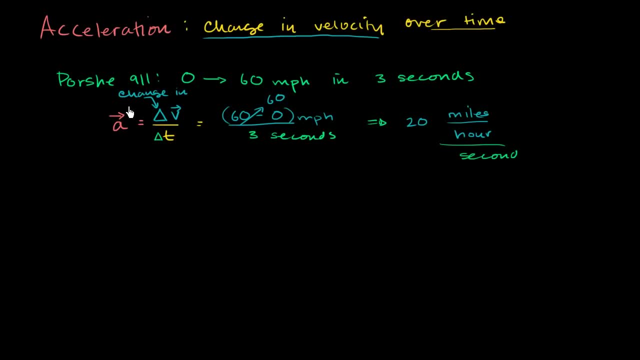 So its acceleration is 20 miles per hour per second, And actually we should include the direction, because we're talking about vector quantities. So this is to the east, So this is east, And then this is east right over here, just so that we make sure that we're dealing with vectors. 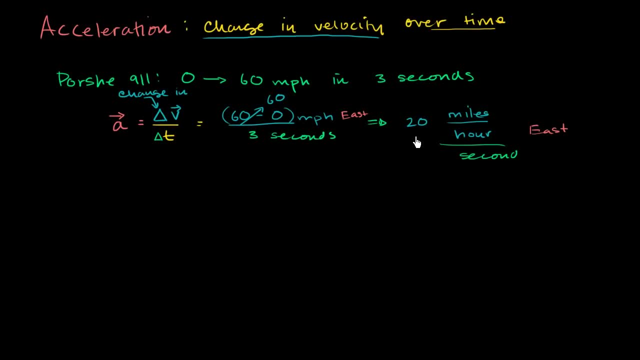 You're giving it a direction due east. So every second it can increase in velocity by 20 miles per hour. So hopefully, the way I'm saying it, it makes a little bit of sense: 20 miles per hour per second. 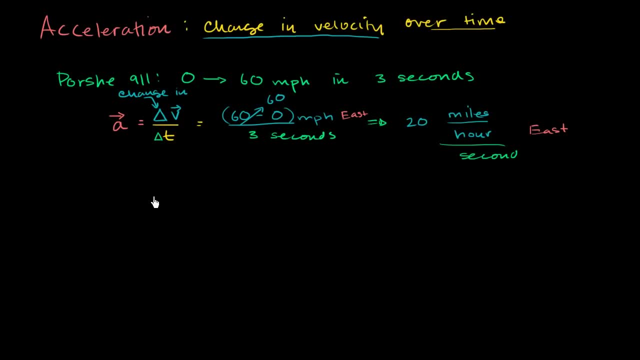 That's exactly what this is talking about. Now we could also write it like this: This is the same thing as 20 miles per hour per second, Because if you take something and you divide it by seconds, that's the same thing as multiplying it. 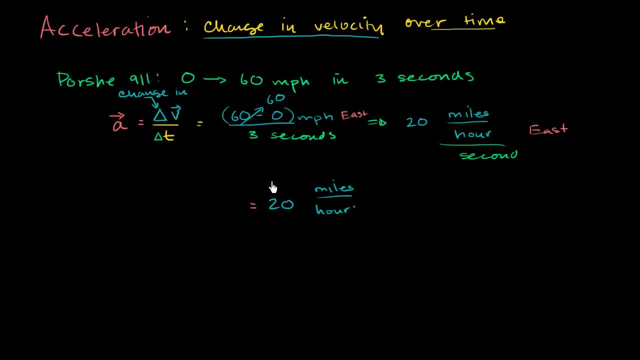 by 1 over seconds, So that's miles per hour, hour seconds, And although this is correct, to me this makes a little less intuitive sense. This one literally says it Every second it's increasing in velocity by 20 miles per hour. 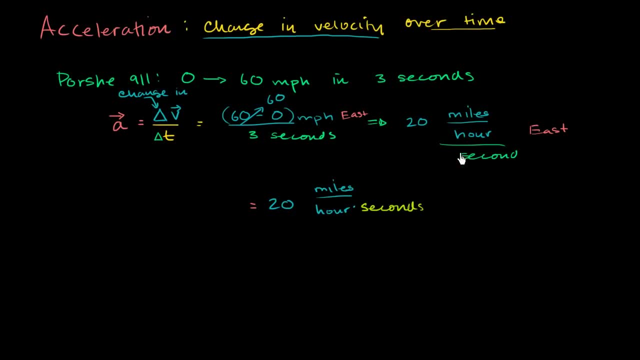 20 miles per hour increase in velocity per second. So that kind of makes sense to me. Here it's saying 20 miles per hour, seconds 20. Once again, it's not as intuitive, But we can make this. so it's all in one unit of time. 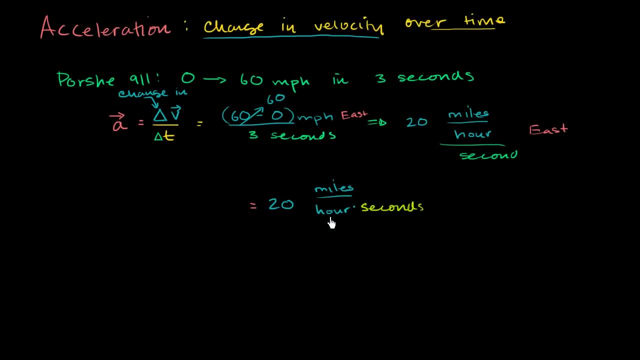 Although you don't really have to, You can change this so that you get rid of, maybe, the hours in the denominator, And the best way to get rid of an hour in the denominator is by multiplying it by something that has hours in the numerator. 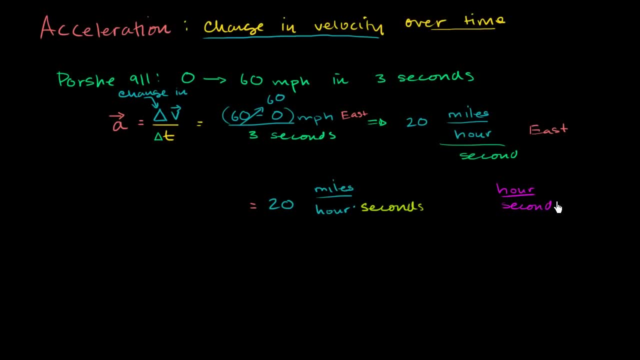 So hour and seconds, And here the smaller unit is the seconds, So it's 3,600 seconds for every 1 hour, Or 1 hour Is equal to 3,600 seconds, Or 1, 1,300th of an hour per second. 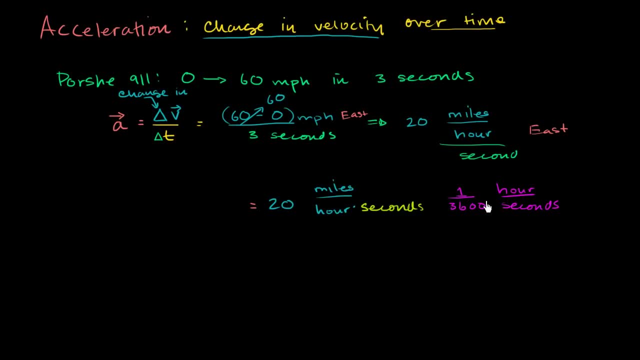 All of those are legitimate ways to interpret this thing in magenta right over here. And then you multiply, Do a little dimensional analysis, Hour cancels with hour And then you have this will be equal to 20 over 3,600 miles. 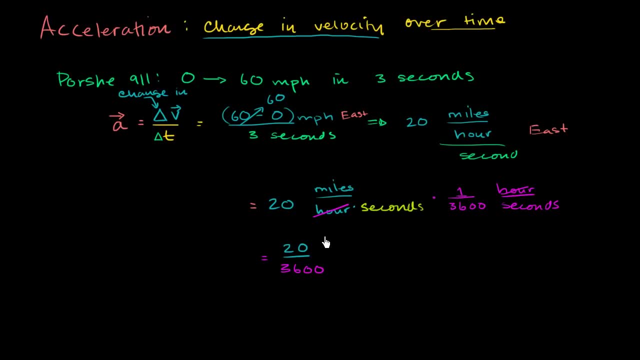 per seconds, times seconds, Or we could say Miles per seconds times seconds, Or we could say miles per second. I want to do that in another color: Miles per second squared. And we can simplify this a little bit. Divide the numerator and the denominator by 10.. 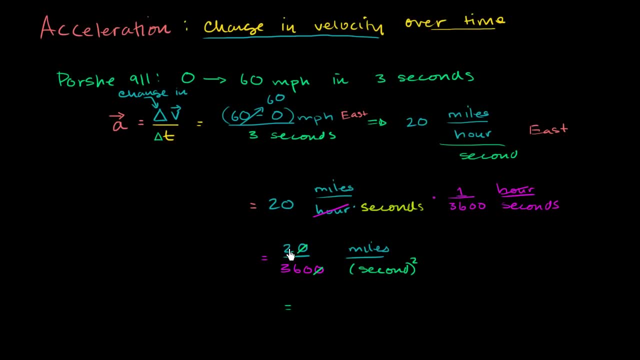 You get 2 over 360.. Or you could get- this is the same thing as 1 over 1 over 180 miles per second squared. I'll just abbreviate it like that And once again, this doesn't make 1 180th of a mile. 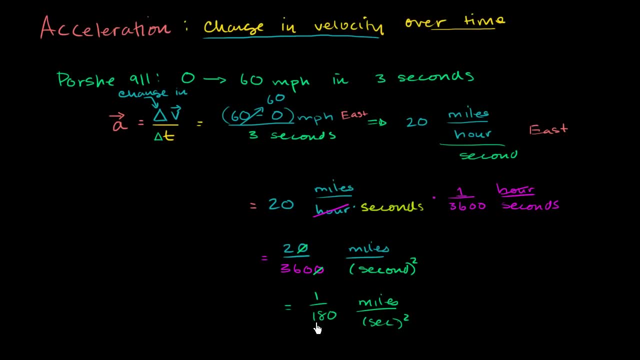 How much is that? You might want to convert it to feet, But the whole point in here is- I just wanted to show you that one- how do you calculate acceleration and give you a little bit of a sense what it means? And once again, this right here: when 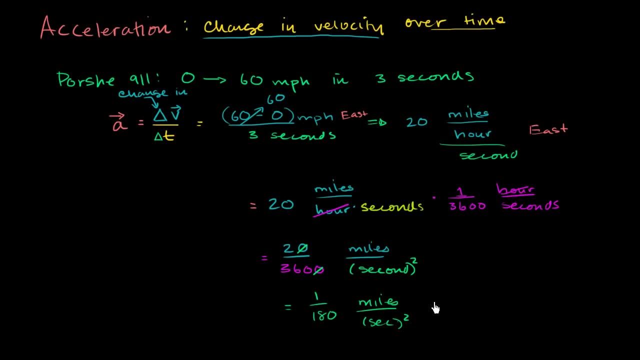 you have seconds squared in the bottom of your units. it doesn't make a ton of sense, But we can rewrite it like that, Like this up here: This is 1 over 180 miles per second, And then we divide by seconds again. 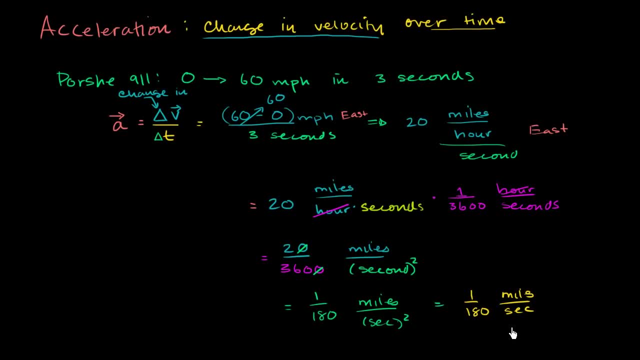 Per second. Or maybe I could write it like this: Per second, where this whole thing is the numerator. So this makes a little bit more sense from an acceleration point of view. 1 over 180 miles per second, Every second. This Porsche 911. 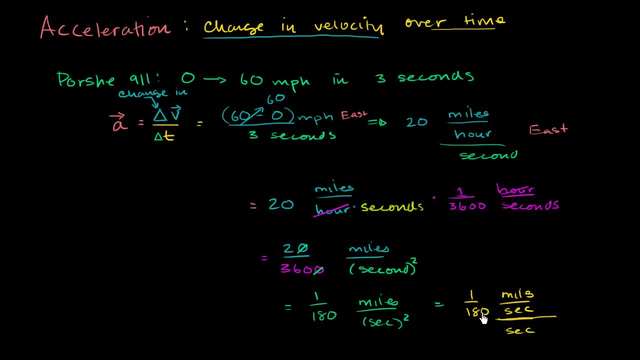 Is going to go 1 180th of a mile per second faster, And actually it's probably more intuitive to stick to the miles per hour, Because that's something that we have a little bit of more sense on And another way to visualize it. 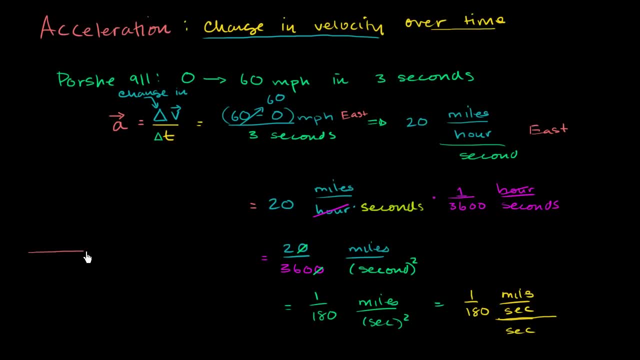 If you were to be driving that Porsche and you were to look at the speedometer for that Porsche And if the acceleration was constant- it's actually not going to be completely constant- And if you looked at the speedometer, let me draw it. 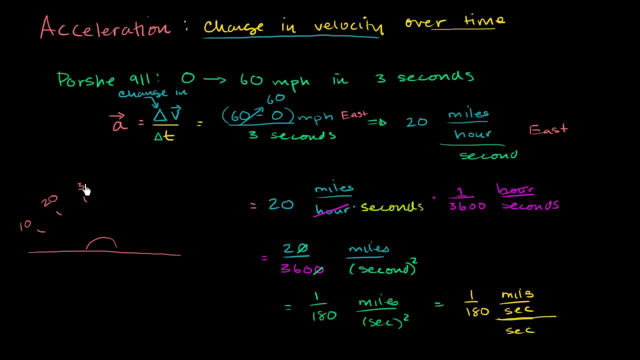 So this would be 10., 20., 30., 40., 50., 60.. This is probably not what the speedometer for a Porsche looks like. This is probably more analogous to a small four cylinder car's speedometer. 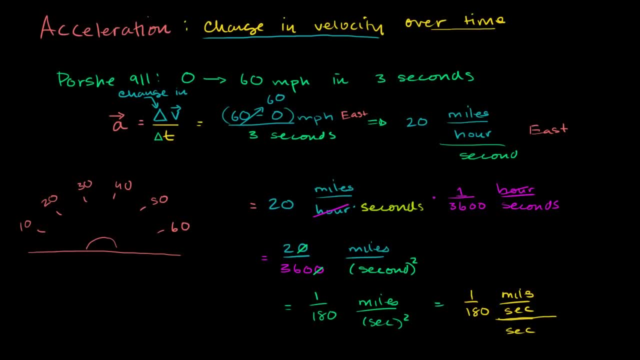 I suspect the Porsche's speedometer goes much beyond 60 miles per hour, But what you would see for something accelerating this fast is right when you're starting. the speedometer would be right there And that every second it would be 20 miles per hour faster. 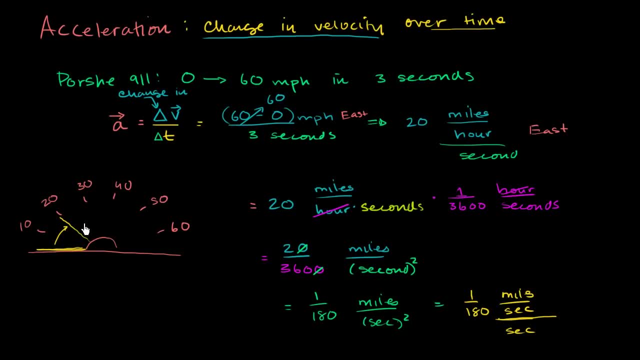 So after a second the speedometer would have moved this far. After another second, the speedometer would have moved this far, And then after another second, the speedometer would have moved that far, And the entire time you would have kind of been pasted. to the back of your seat.